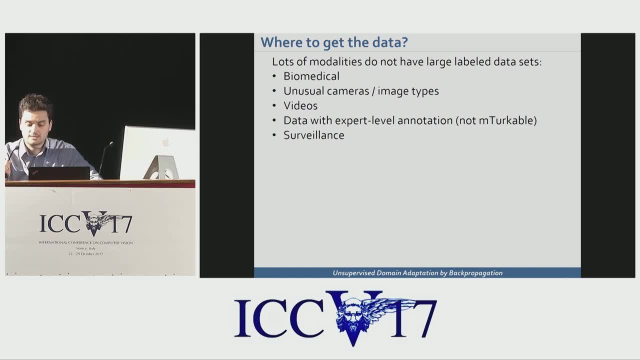 is challenging for humans, especially for non-experts. There are also many tasks requiring pixel-label annotations, and such annotations can be really tedious. So in such situations there are often some sources of surrogate data, and exploring those sources becomes more and more popular in the community. For example, one can borrow from: 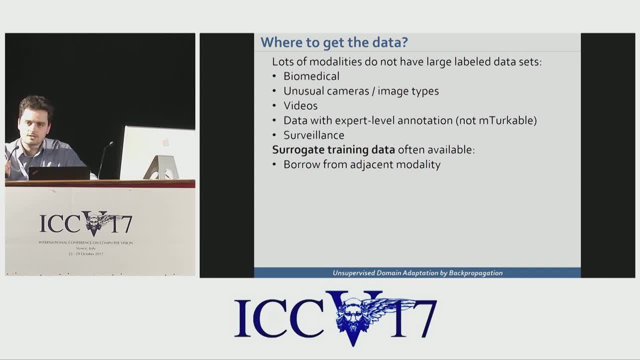 adjacent modality, having similar but different images which are annotated. One can generate images using computer graphics And finally, in many cases, one can use the computer graphics to create a lot of results from the data that one has already acquired. This would give you a big annotated dataset. but unfortunately, in many real-life situations 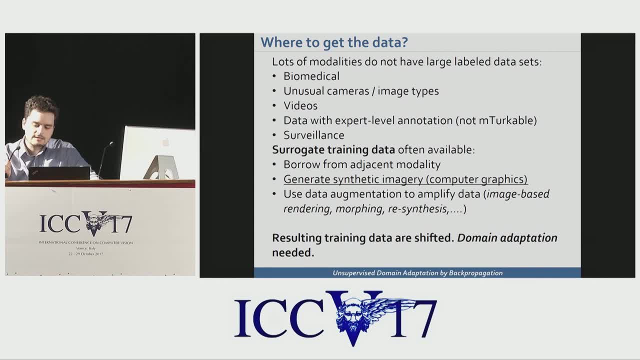 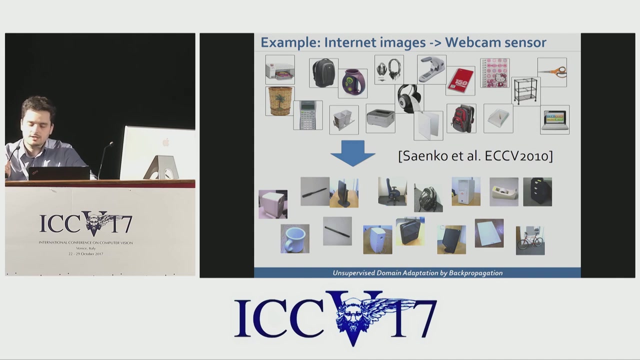 the resulting training data is shifted in a certain sense and deep networks trained on such shifted data may overfeed to the differences between the training data and the data you actually care about, leading to quite significant drop in performance. Just to give before I proceed. just to give you some concrete examples. this is an illustration. 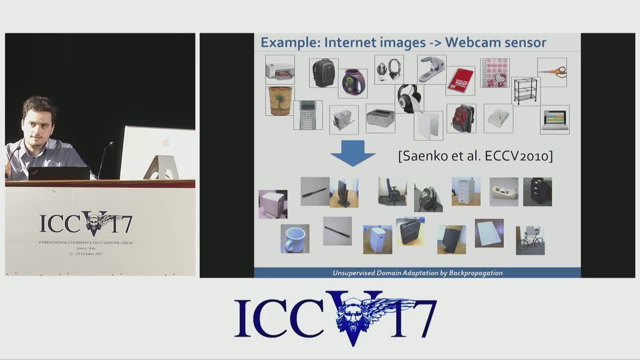 from the most popular benchmark of such multiple domain training, the Office dataset and this particular pair of domains of image types, shows the realistic scenario when you train on internet-originated images and you want to deploy your image classifier, say, on your. 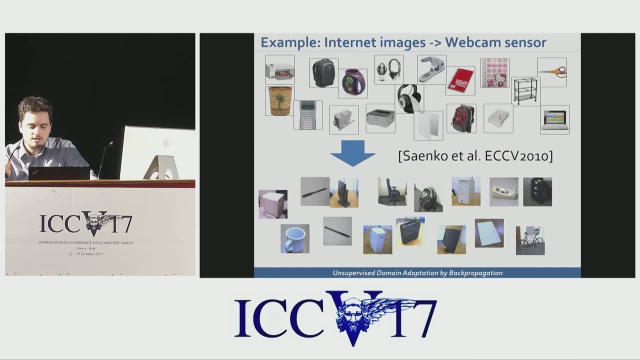 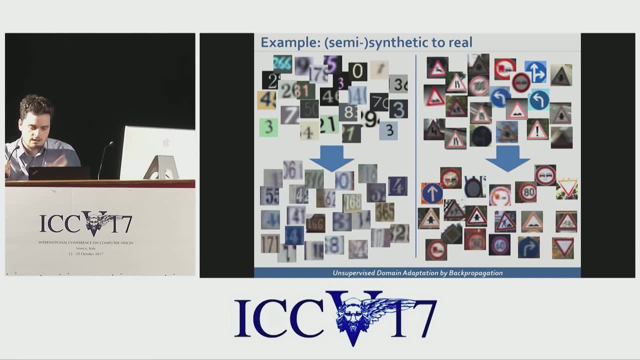 robot which is equipped with something like a webcam, and you see that the images look really differently, even though they depict the same classes of objects. Another popular scenario: you train on synthetic data, like on the left, or you train on semi-synthetic. 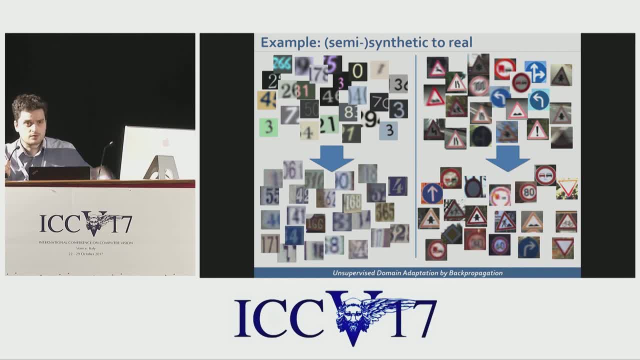 data, and I call it semi-synthetic because it uses real backgrounds, Okay, And the real image is simply placed on top, but the simple imposition process is artificial. And then you want, of course, your trained network to perform well on real data. 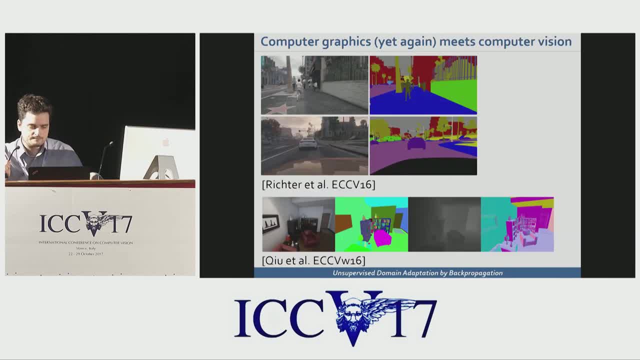 And this synthetically-generated data training is becoming really more and more popular. Here are some illustrations from two very recent work and you see images which look really realistic and they are meticulously annotated. You get this. You see those pixel-level annotations which would be really hard to get with human labeling. 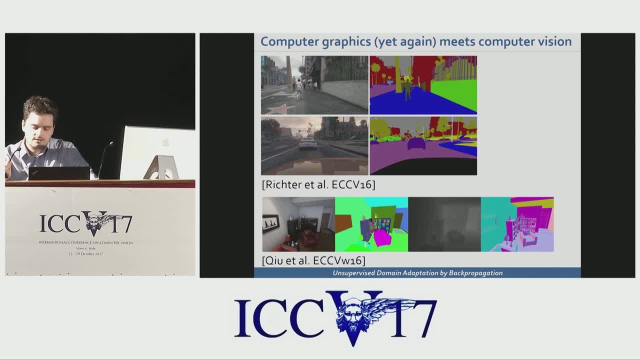 But unfortunately, while those images do look realistic to us, the results of network training just on them are actually quite poor. So to get the really good results, quite a large amount of labeled real data have to be admixed into the training process. 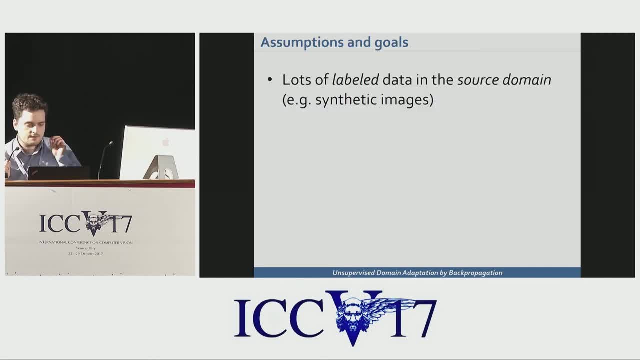 So today I will consider the following, The following: Okay, Let's assume that you have lots of labeled data in the source domain, like synthetic images. Let's assume that you have lots of unlabeled data in the target domain, for example, real. 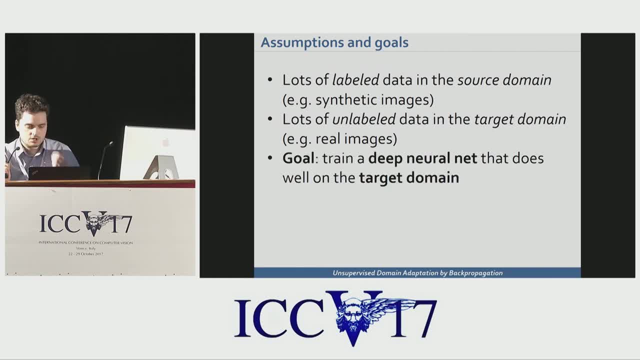 images And your goal is to train a deep network which does well on the target domain. Such scenario is called unsupervised domain adaptation. There could be cases- and maybe in most scenarios there would be a case- for semi-supervised domain adaptation, when you have some small amount of labeled data in the target domain. 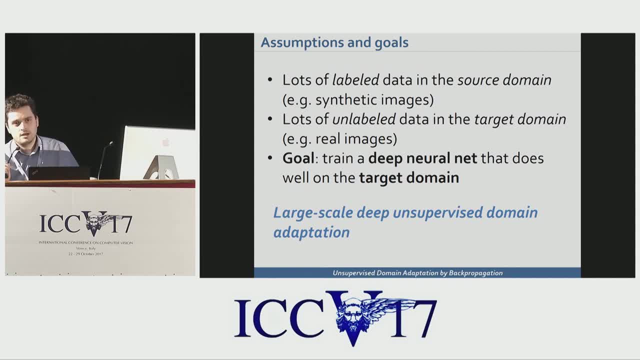 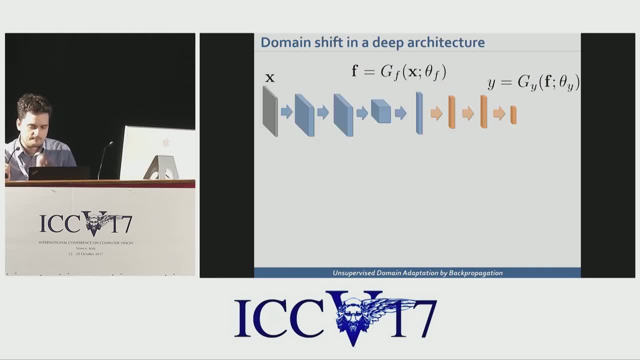 But the ideas I will be talking about today generalize to those scenarios pretty straightforwardly. So the problem that we will be dealing today is the difference in the two distributions. To highlight this difference, let me take my deep network and let's assume it was trained. 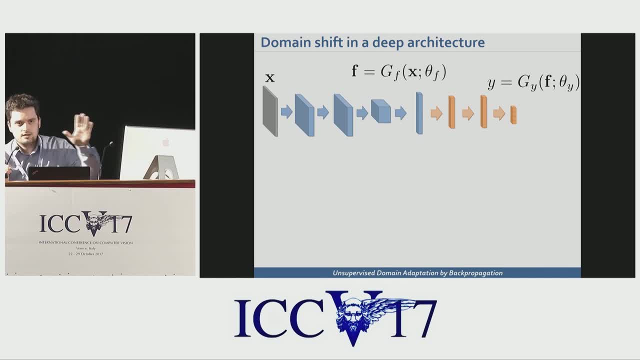 on a source domain. So I will split it into two parts. The first part I will somewhat arbitrarily call feature extractor and the second part I will call level predictor. Generally, I will be talking about image classification for the most part of the talk, and then I 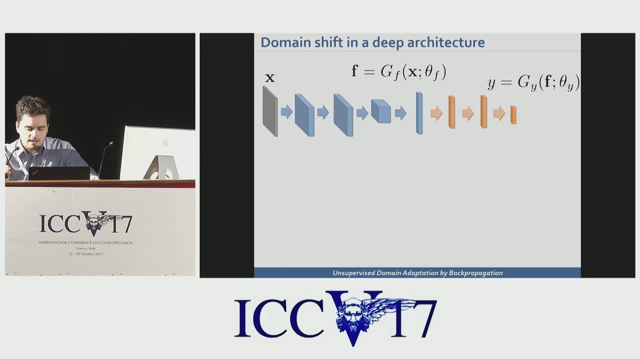 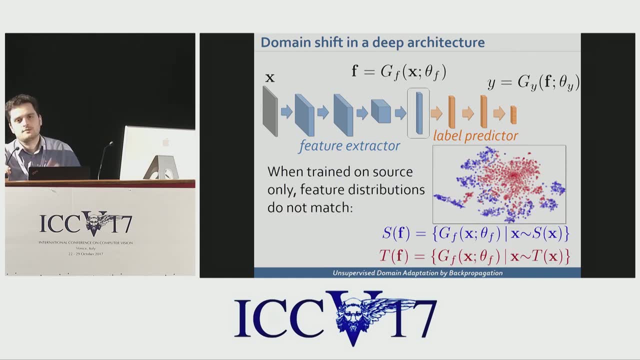 will discuss other tasks And then it will look at the visualization of the features extracted by the feature extractor. And if I look at what are the features of the two domains and I'll show them using tcne encoding: Okay on a plane and red would denote the target domain and blue would denote the source domain. 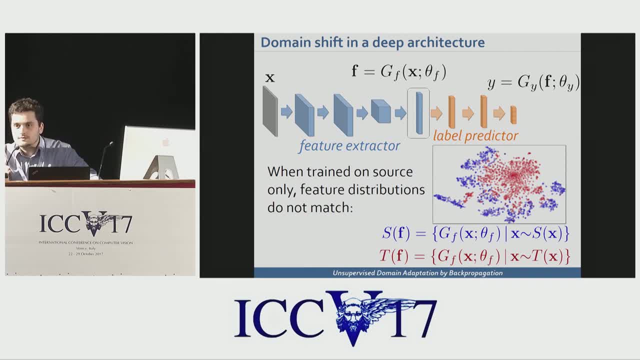 what we will see is that the two distributions are really different. This is actually a real case example for some real data sets. The blue features are already nicely separated by the time we get to this middle of the network and those groups correspond to individual classes, while the red distribution is quite complex and distinct from the blue one. 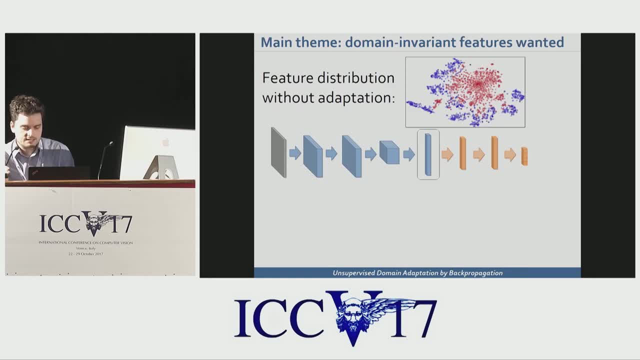 So what we need is some mechanism that would allow us to align the two distributions. We want to get to this situation where blue and red features are distributed approximately similarly and then blue features are still good for classification. So we need some mechanism to perform alignment. 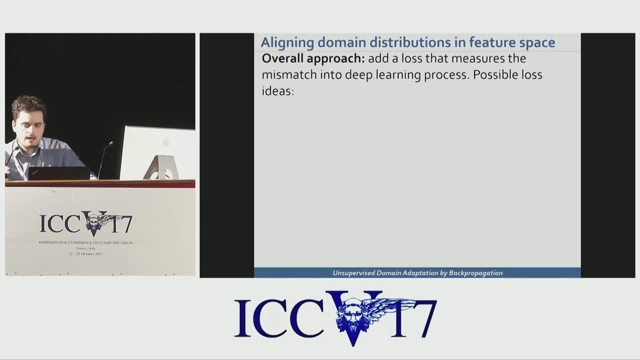 So we need some mechanism to perform alignment. So we need some mechanism to perform alignment of distribution in high dimensions. and there are many way or several ways how you can do it. with deep learning generally, you take some loss which measures the separation between distributions and you plug it into the learning process so that during learning it affects. 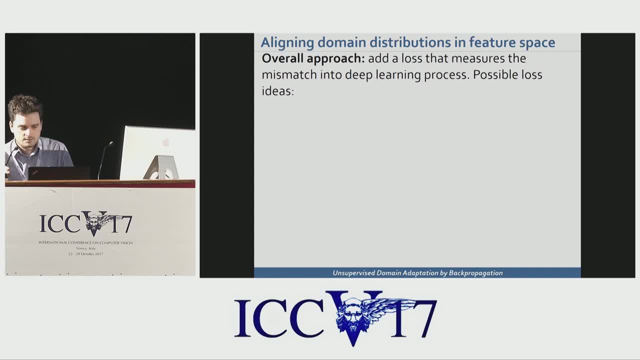 it affects the feature structure and possible choices are: um, do it parametrically, like measure first and second order moments, and that would be your loss and you want to minimize it. so you want to align your distributions up to those moments and this has been tried for domain adaptation in this work and some others. another popular idea is maximum. 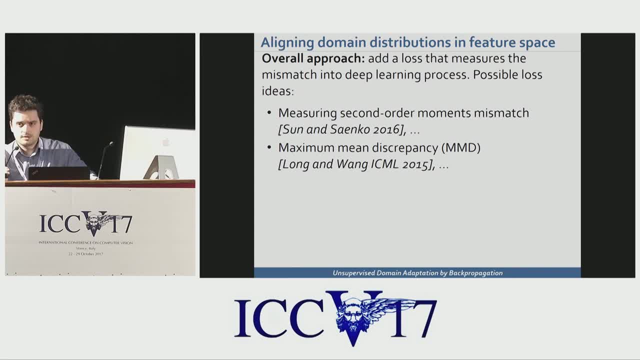 mean discrepancy, which has already been investigated and works well. today i will naturally be talking about adversarial learning for distribution alignment guns can be used for for distribution alignment, as has been already discussed, and that's how we'll use them here in the first part of the 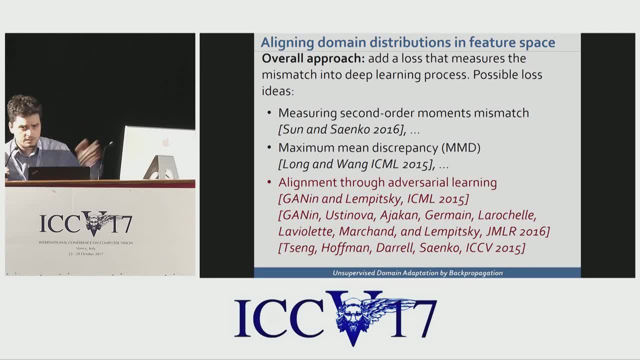 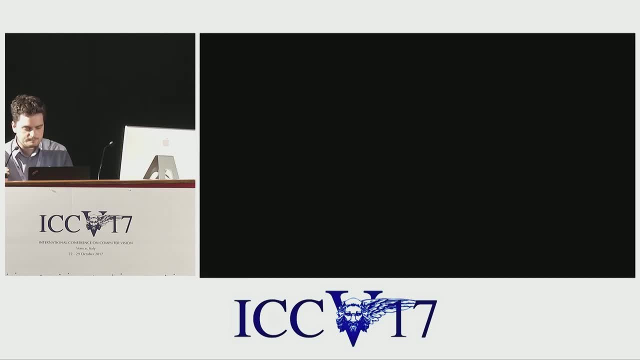 talk, so the results will be from mostly. the first two papers here- and many of them will be- were obtained by yaroslav ganin, who is my pg student. okay, and now we have a problem. ah, yeah, um, i haven't touched anything. i can try to replug. 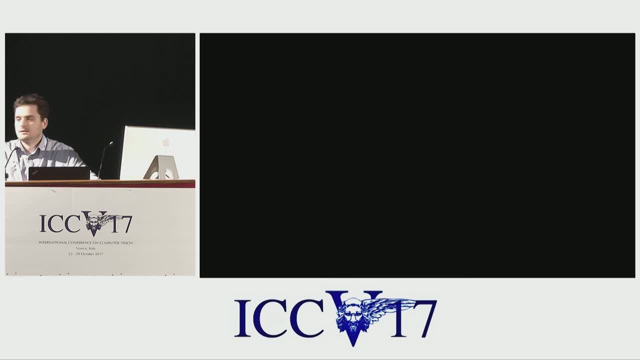 uh, the projector is not working from what i can see here. Hello, Houston, Can someone in the back, May I take help from technician? Okay, that's better, thank you, Okay, Okay, Thanks. So now, since we want to do adversarial learning, we will start by adding a binary classifier. 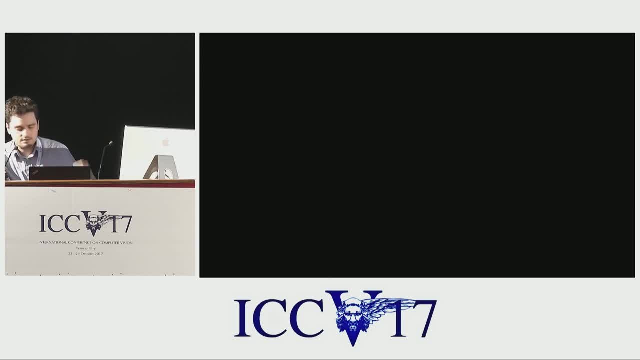 a domain classifier, which will look at points in the feature space and try to predict, will be updated to predict which domain would they come from And, in the situation when the two distributions are easily distinguishable, the domain classifier will be able to distinguish between them. 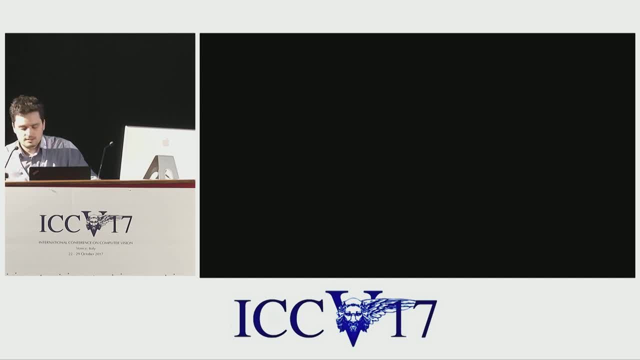 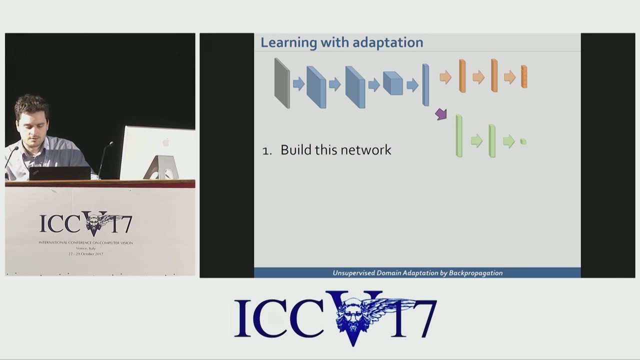 So both the main classifier loss will be low and when they're mixed it will be high. So we want a feature extractor to fool the domain classifier and to ensure that its loss is high. So what we'll do then? we'll build such a tripartite network and we will train the feature. 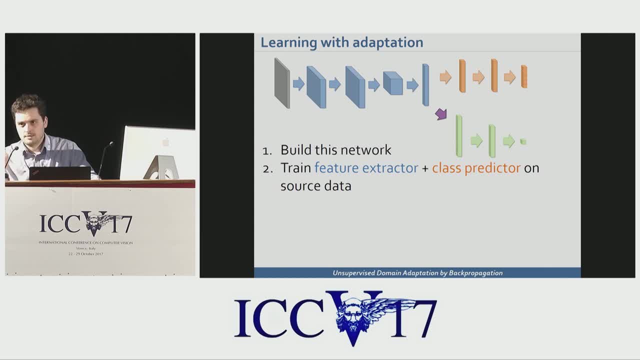 extractor in class-predicted on source data. because we need labels for such training and we only have it for source domain And we will train feature extractor, feature extractor and domain classifier on all data because we don't need the labels, we just need to know which domain does each example come from and at test. 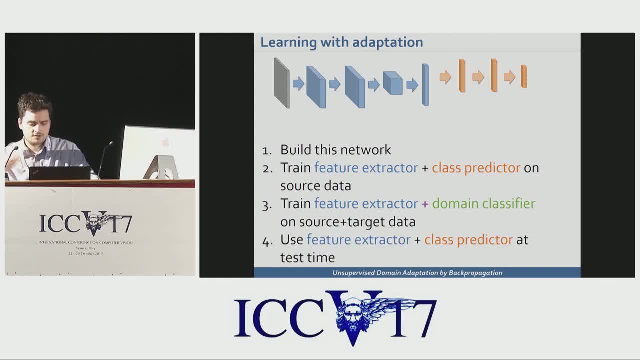 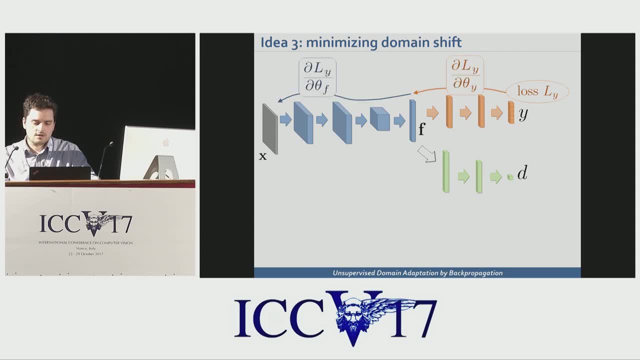 time we will just discard the domain classifier and use the feature extractor and class predictor to make predictions. here is how gradients will flow in this during the learning process using standard back propagation. so the feature extractor will be updated by the losses both from class classifier, class predictor and the main classifier. and if I just do this naively, I will get 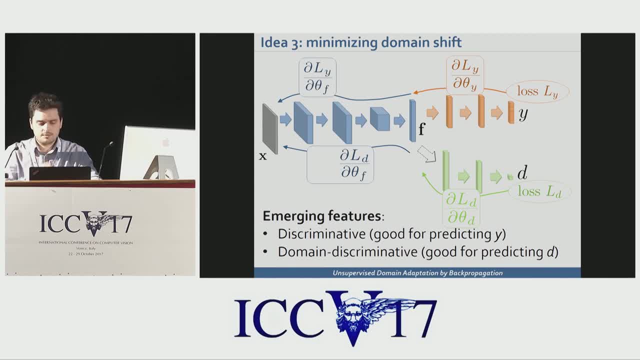 features which are good for predicting class labels but are also good for predicting predicting domain label. that's, I want the first one but the opposite of the second one, because I want my features to be domain invariant in this setting. so what I can do is I can use the class predictor and class. 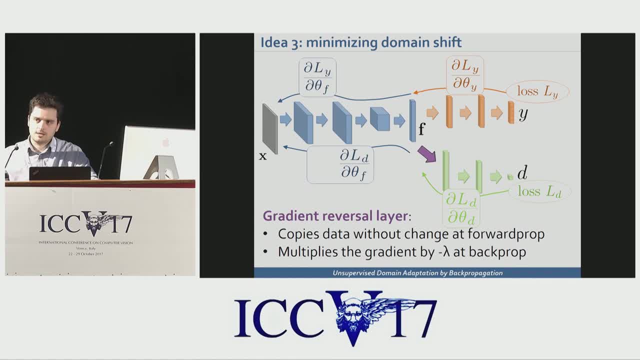 predictor. I can do. the existing I can do is I can reverse the gradient when it comes during back propagation from the domain classifier into into the feature extractor, by multiplying it by some small negative constant and then, if the learning process is successful, I will go to features, I will get features. 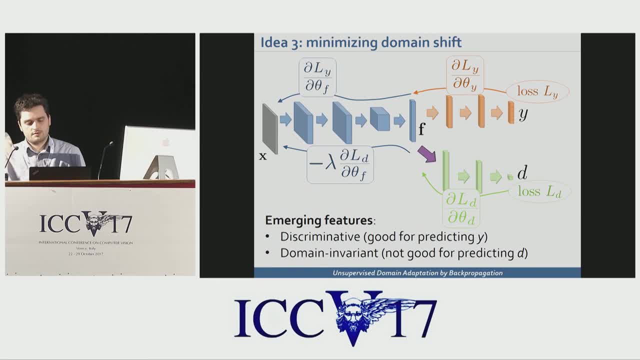 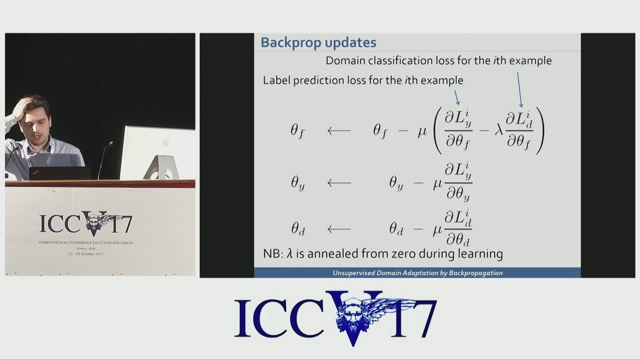 which are a domain invariant, at least from the viewpoint of my domain classifier. okay, that's the idea how we proceed. these are some four formal equations, for the main, for gradient descent. of course we can use like Adam version of that. one important idea is that you have to anneal those. 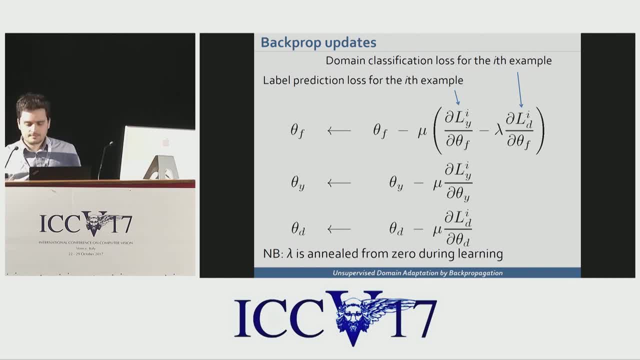 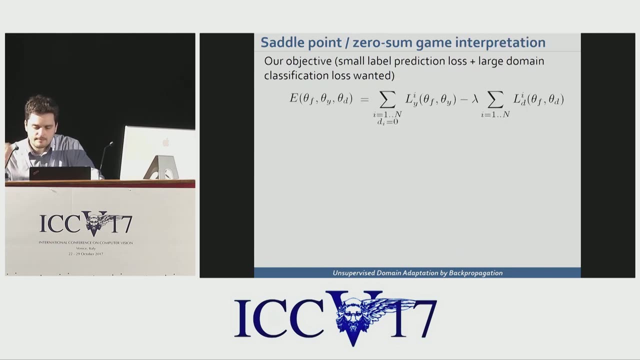 lambda, this lambda, from zero to something constant, because during the early stages, having this adversarial term really confuses the training process. okay, now if we analyze where does this process leads, and then we can see that if it converges, then it converges to a saddle point of zero sum game, with this policy played with, played by. 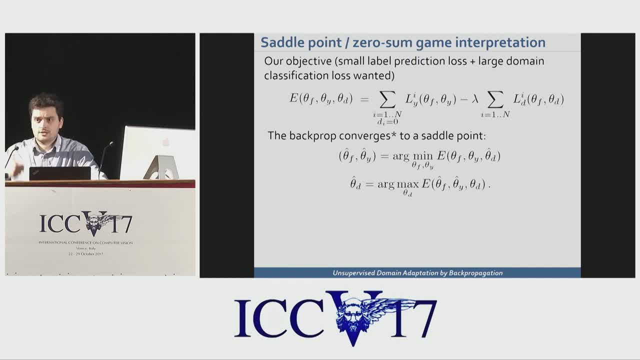 domain classifier on one hand, and feature extractor and label predictor on the other hand, and so this is zero sum game. we have also tried a non-zero sum game Using Claiborne inversion. this is trick number two from Sumitha. talk before the lunch break. 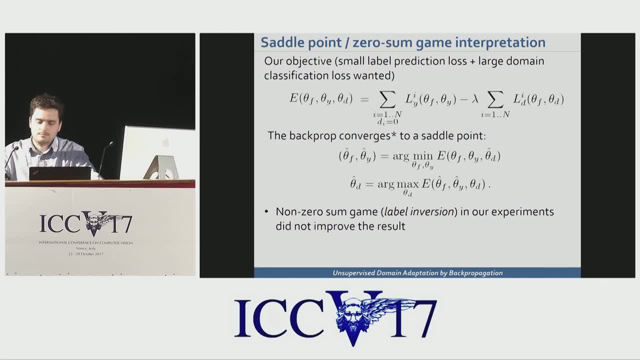 In our experiments. it did not improve the results, but it may be still worth trying. In parallel with us, Berkeley group investigated the same idea and they found out that in their experiments, especially in the early stages of training, the maximum confusion. 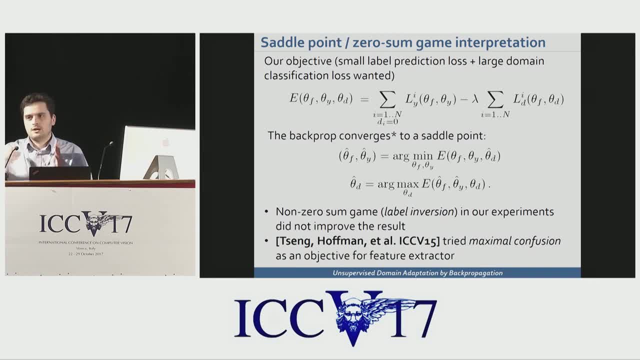 objective which measures used for the feature extractor part worked better And maximum confusion means that they measure cross-correlation with the cross-entropy. with 50-50 distribution, The feature extractor is updated so that the discriminator thinks that it has equal chance of coming from source domain. 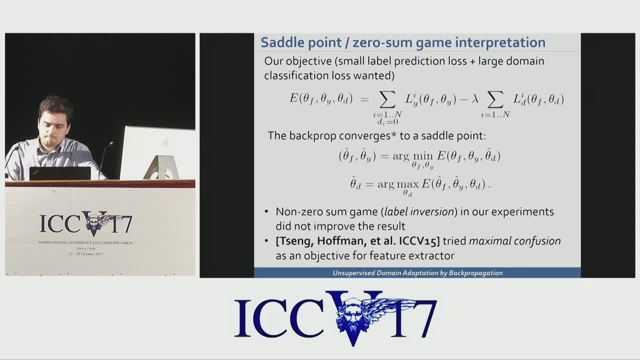 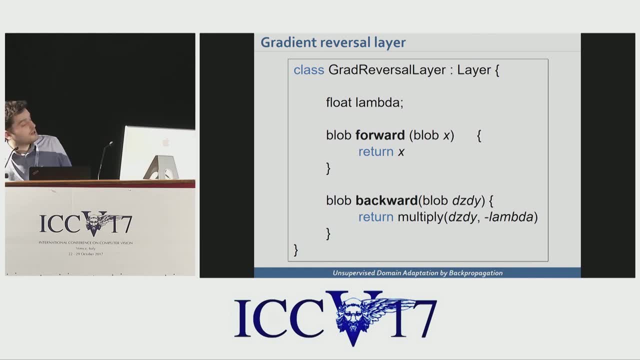 and target domain. OK, If you go for the simplest case, the zero sum game, then you can implement it using this gradient traversal layer, which is easy in most deep learning packages, And then you can train your discriminator, your domain classifier and feature extractor. 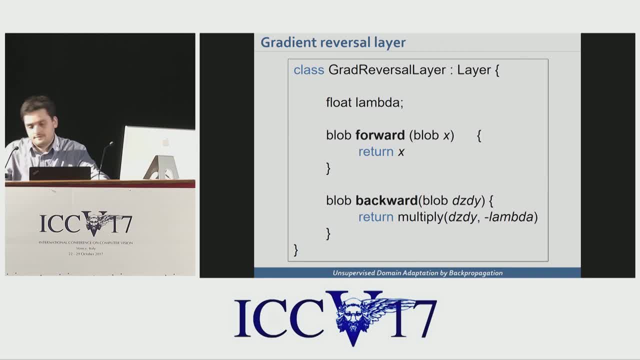 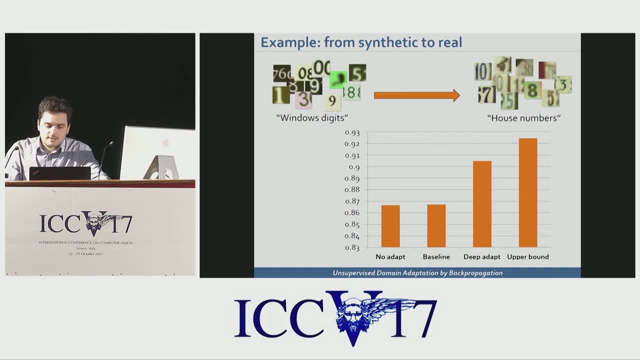 at the same time, not in stages, which can have slight benefits, But of course you can do it in stages like in normal game training. So does it work Well in some situations this approach does. This is one example. 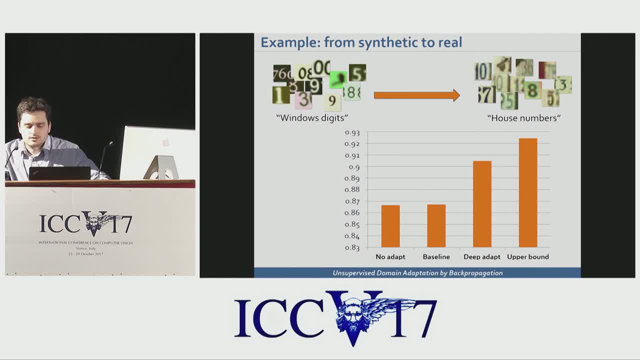 We train here on synthetic digits and test on real digits. The no adapt column is what happens when you train on synthetic data and just test it on real data without any changes. The upper bound, which is perhaps not exactly correct, but anyway, upper bound here means 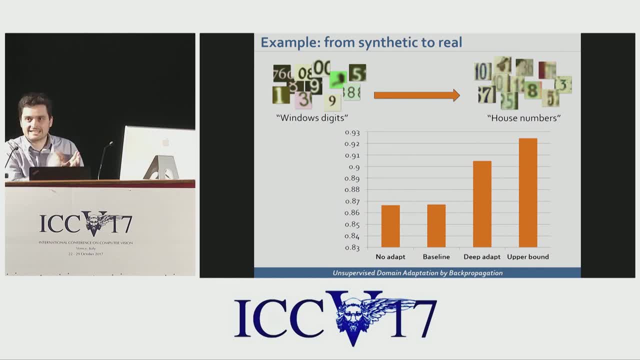 a system which is trained on real data and that has access to the labels in the real domain. And deep adapt is the approach that I have just discussed, which doesn't have access to such labels, but has access to unlabeled data in the target domain. 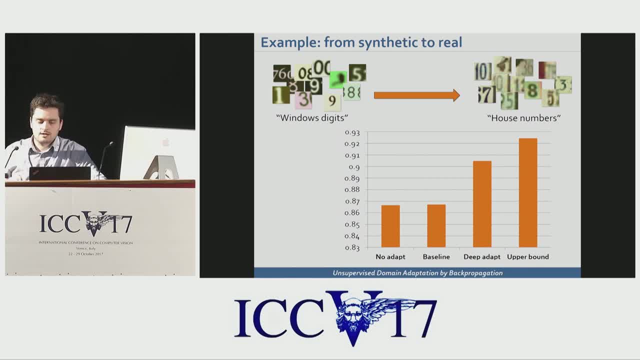 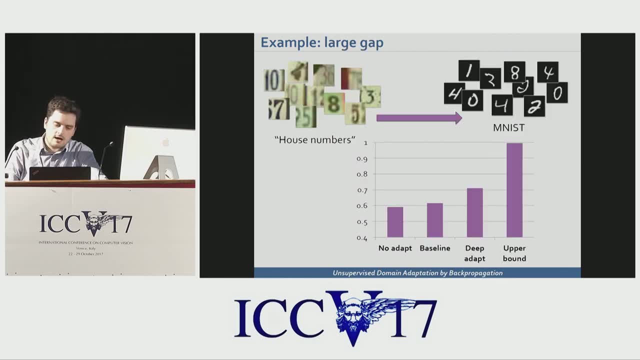 And in this particular case, it bridges this gap between no adapt and upper bound, bridging the majority of this gap, This situation, it's less successful, but still we see considerable improvement. Interestingly, when we look at the reverse direction, it doesn't work. 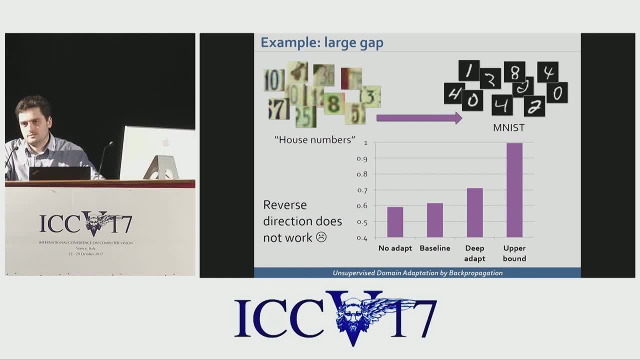 Well, it works. It works better than chance, but it gets maybe to 30% or so, which is quite low, And I think the reverse direction is a good benchmark for methods. I think it's still very few methods managed to make it work as of now. 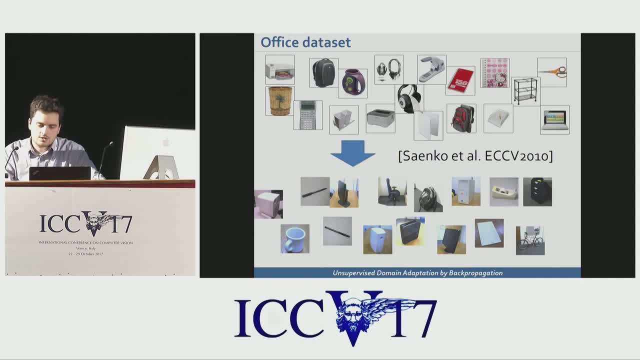 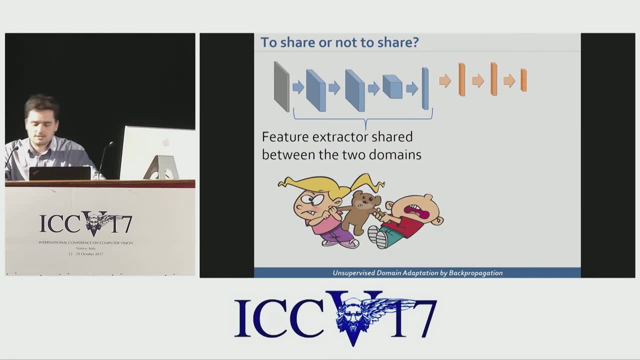 We also tried it on the office data sets and got results which were state of the art as of two years ago, But since then they were superseded by newer methods that I will discuss now. OK, So one potential source of improvement is not sharing all of the feature extractor. 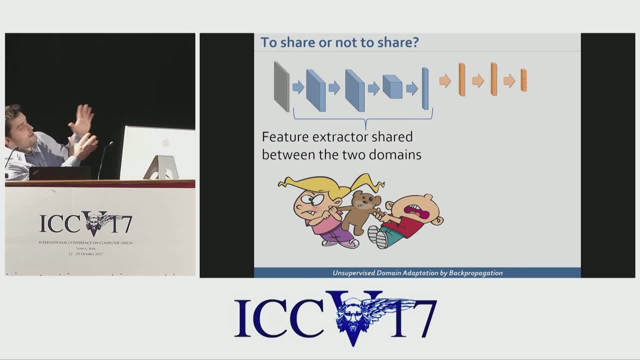 between the two domains. So far, in the project I discussed, same feature extractor was used for both domains And we discussed at some point in our group whether this is the right thing to do. I was insisting: yes, it was the right thing. 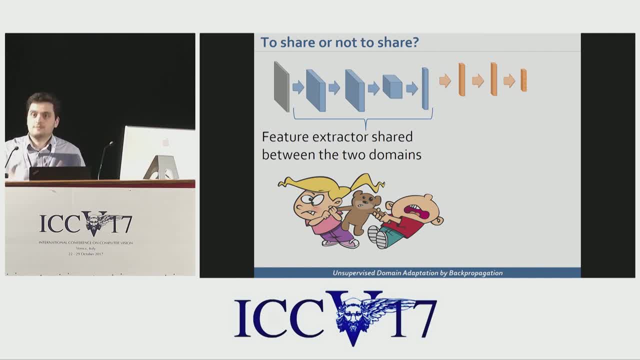 Those feature extractors are very big, They have tons of parameters, So they should be able to learn good feature matching, which is both feature matching, Which is both invariant and extracts all necessary information which is required for classification. Turns out I was wrong. 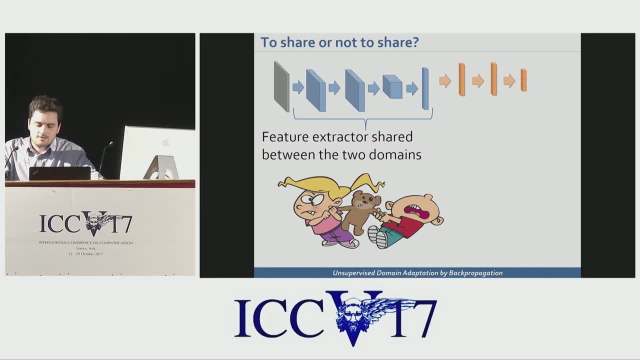 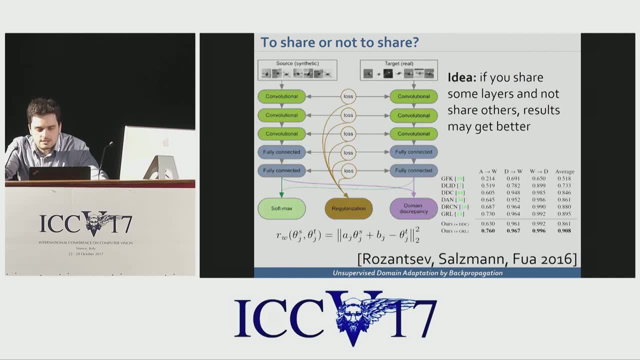 And you can do better by training two separate feature extractors for each of the domains, But you have to do it carefully. One example is this paper, which showed that by sharing parameters in some layers but not sharing in others, you can get better. 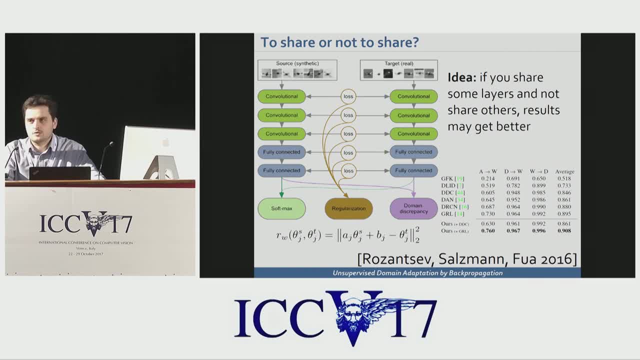 Better results. But when you don't share, you have to have some regularizer which penalizes the difference in weights between the two domains. For example, it ensures that the weights in one domain are close to some fine function: constant time plus bias. 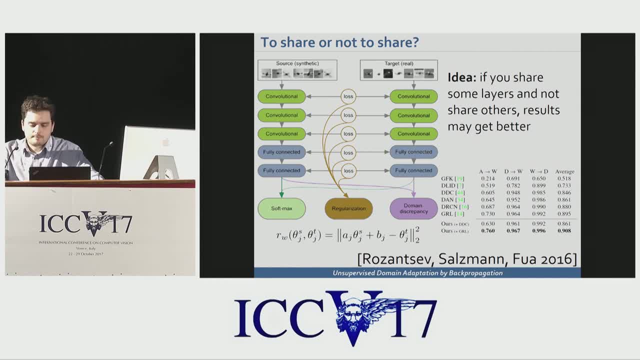 of the weights in another domain. And then you have to use some criterion to decide which parameters to share and which layers not to share, And unfortunately in their experiments there is no consistent strategy. You have really to decide it on a case-by-case basis. 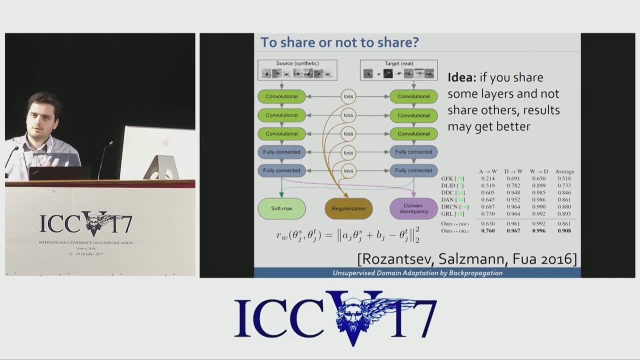 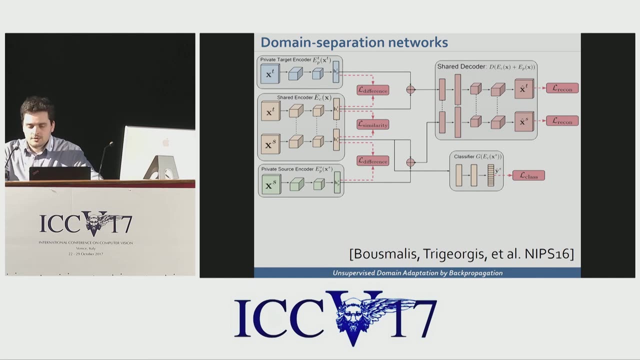 So for some domain pairs some layers have to be shared, but not for others. So this is a challenging task to accomplish, But if you do they get quite significant improvement in the results. Domain separation networks presented by Google Group last NIPS went further. 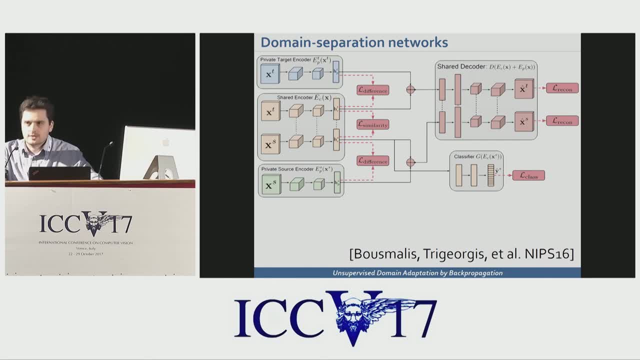 Here they have a system which, as you can see, can perform classification and reconstruction at the same time, And they train three different feature extractors: one which is shared between the domains, and the other two are not shared, They are domain-specific. 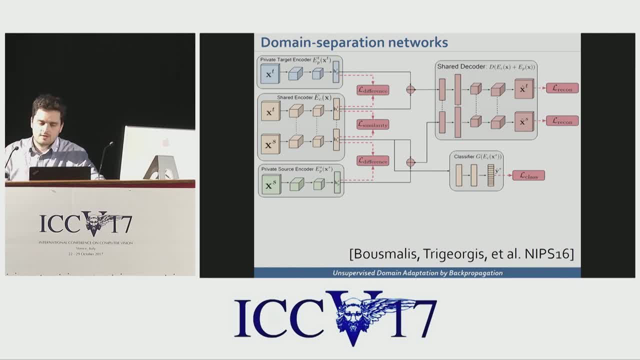 And the shared decoder has to be able to reconstruct the original input data. And then there is an adversarial term, just as in the previous approaches, which ensures that the features extracted by shared feature extractor have similar distributions across both domains. So that's inherited from the previous approach. 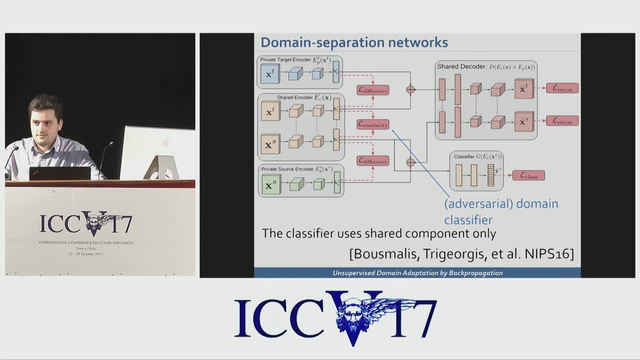 And then, of course, your classifier has to make classification based only on the shared features And, by construction, ignores domain-specific features. And the last bit which is required to make it work is some regularizer which enforces orthogonality. 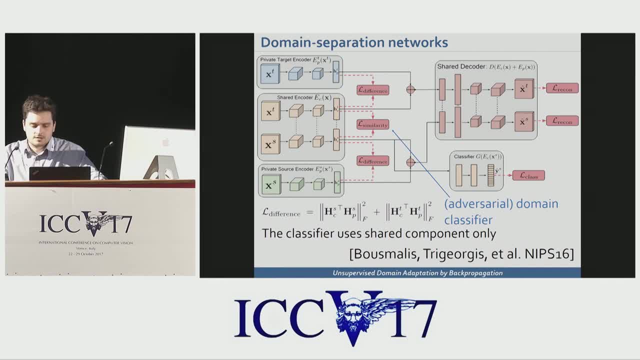 between shared features and domain-specific features, And they have shown that with this architecture, which combines this auto-encoding orthogonality and adversarial learning and classification, they can get quite significant improvement on a range of data sets. OK, and then the last approach. 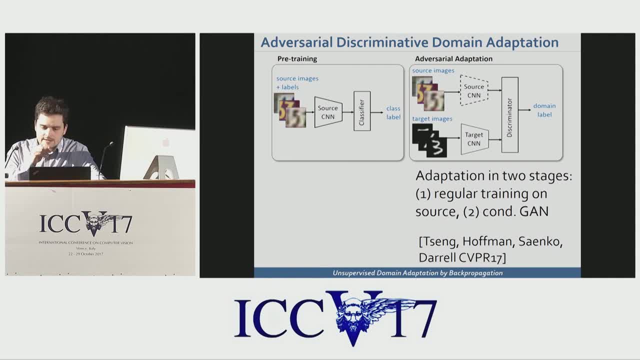 I want to go in some detail today is the recent work from Berkeley and Boston Groups, which is another very nice twist of the adversarial domain adaptation. Here they do it in two stages and they show that it works better than when you do it in one stage. 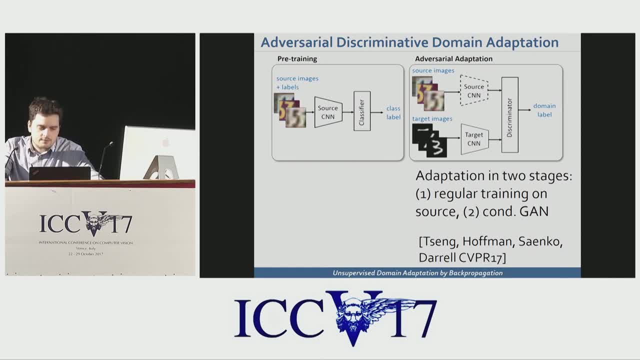 And the first stage is straightforward: training of classifier. OK, So a class predicting CNN on the source domain. So we just train a regular predicting on source domain, no twists. And then in the second stage you freeze what you have trained in the first stage. 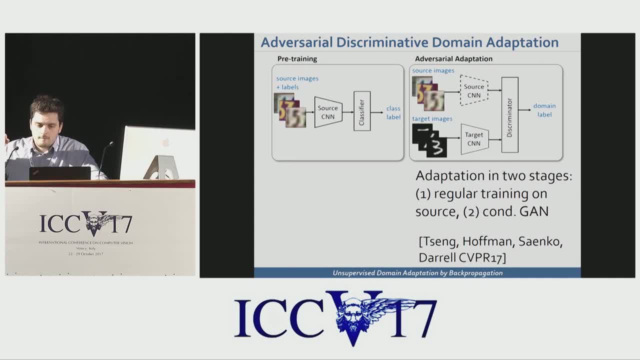 So we get some fixed feature distribution for source domain And now you train a new feature extractor which is essentially conditional generator for the target domain And the goal of training is to learn a feature extractor which would match the distribution of the source domain features. 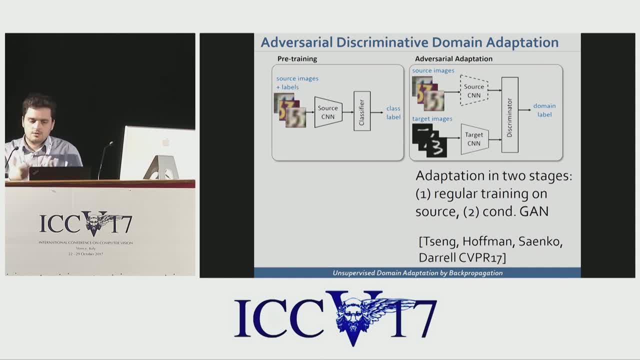 So essentially this part of the training, this stage, corresponds to adversarial learning conditioned on the input images, where you match distribution in the feature space And then at test time you just use a new feature extractor and a classifier And that's the classifier from the first stage. 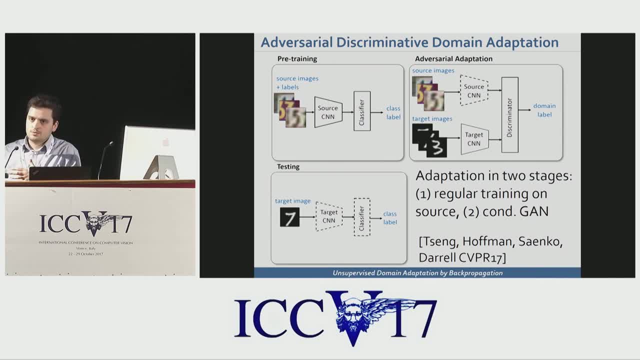 And I think this breaking into the two parts makes it easier to train, especially if you're familiar with generative GANs. then you can use your experience in training over the second stage of the approach. OK, So I've been talking almost exclusively. 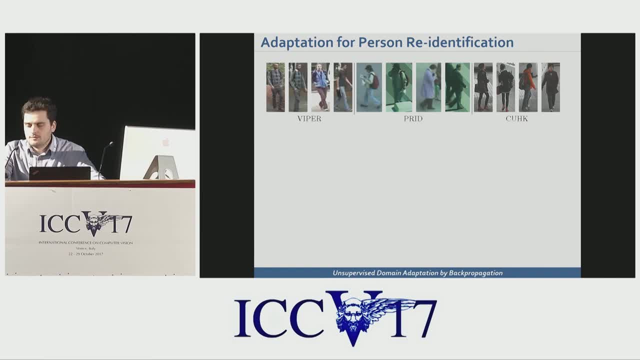 about classification and I probably won't have time to go into detail on other tasks. But I just want to mention that you can use very similar ideas for other computer vision tasks, For example in re-identification, where domain shifts are a big problem. all those data. 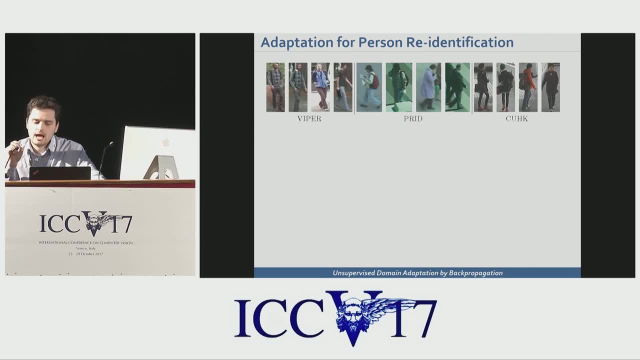 sets, they have different looking images and a limited amount of annotated data. So annotated data is precious. And then if you combine metric learning with domain adversarial term, just as in the classification case, you do get this small improvement in re-identification accuracy. 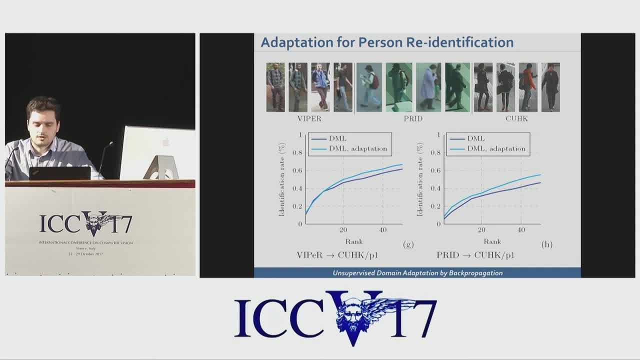 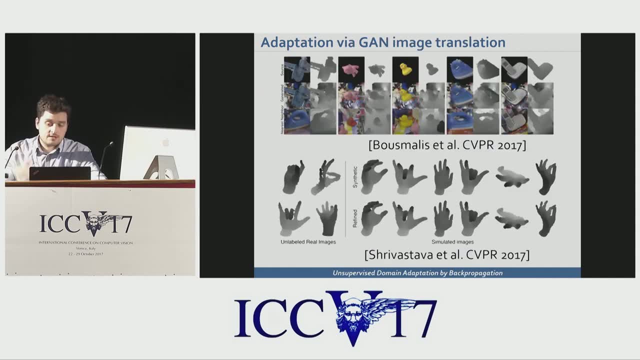 There are also other works that show that- for semantic segmentation. Finally, before I come to conclusions, let me mention that there is another string of work which is not covered in this talk, but we just have a little bit of time, OK, So one of the things that is becoming increasingly 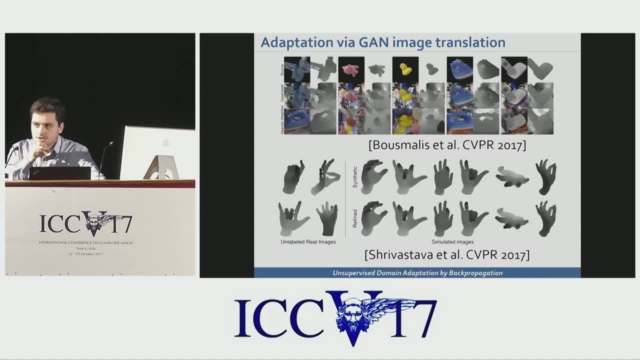 popular when you use adversarial training to do domain adaptation, but you don't adapt at feature level, somewhere deep by matching distributions, somewhere deep in your network, And instead you use GANs. you use generative GANs to translate, to modify, say, your synthetic images. 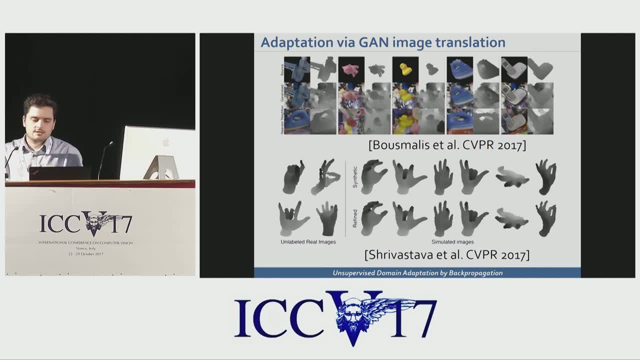 to make them look more like real, to add some artifacts typical for real images, And they show both of these works, let's say from, but there are more examples show that this works, although mostly they showed that this works for quite closed domains. 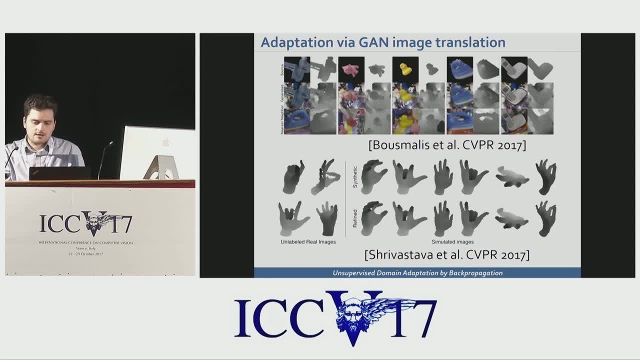 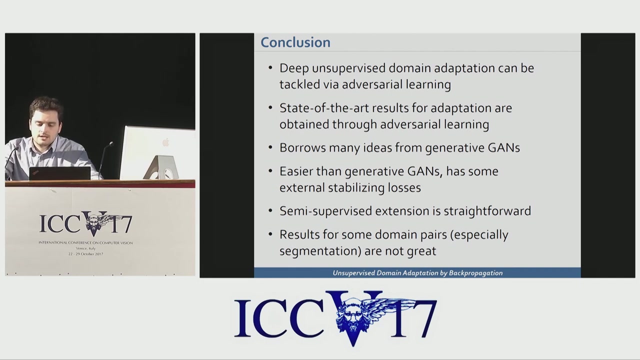 OK, I cannot say anything conclusive, but the intuition is that for large domain gains it makes more sense to adapt in feature space. But of course intuition can be deceiving. OK, So to conclude, unsupervised domain adaptation can be handled using adversarial learning. 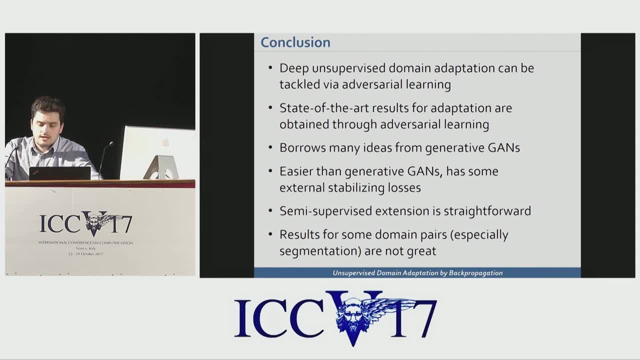 Extending to semi-supervised case is straightforward. This process borrows ideas from generative GANs, but it is in some sense easier because you always have some external loss and other loss which stabilizes the training, at least to some extent. 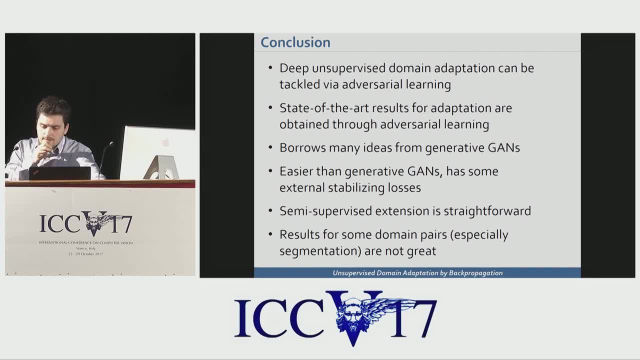 What's challenging, though Well, another benefit compared to generative GANs is that you have real numbers. how to judge your success? which are numbers? how does your system perform on target domain When you do unsupervised domain adaptation? that is like a big caveat, though. 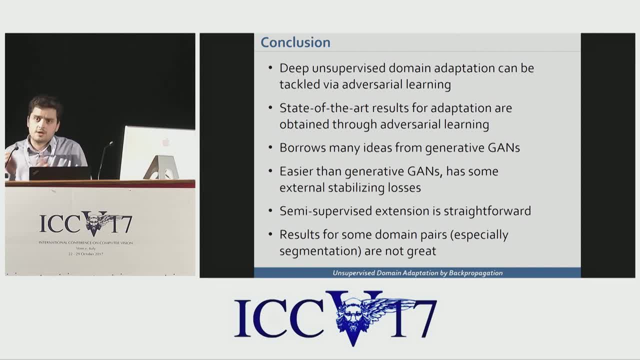 Currently working with GANs requires lots of parameter tuning And when you do unsupervised domain adaptation, once you for the first time look at your performance of your system, your test set, then parameter tuning essentially becomes cheating and you have to walk this fine line. 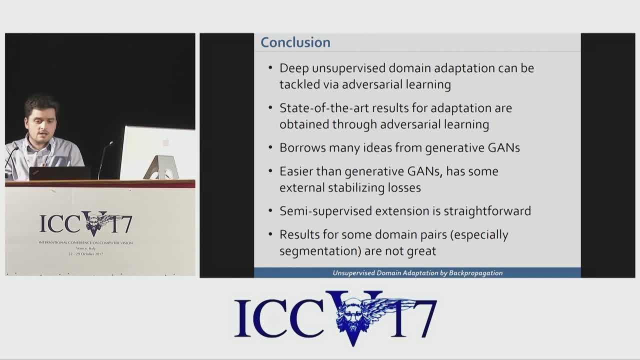 So this is, I would say, the main challenge here, And another thing that I wanted to mention in the end is that I've shown you some examples and excerpts from some papers which report really good results, but it's definitely not a solved problem for some domain pairs. 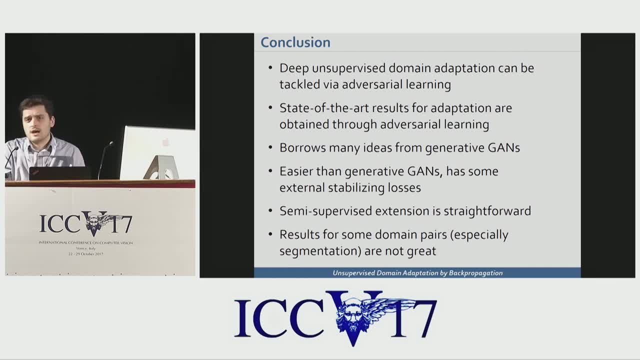 and some tasks, especially for semantic segmentation. I would say The results for unsupervised domain adaptations are actually quite poor and there are lots of gains to be made, So there should be definitely new development in this story. Thank you for your attention and I think